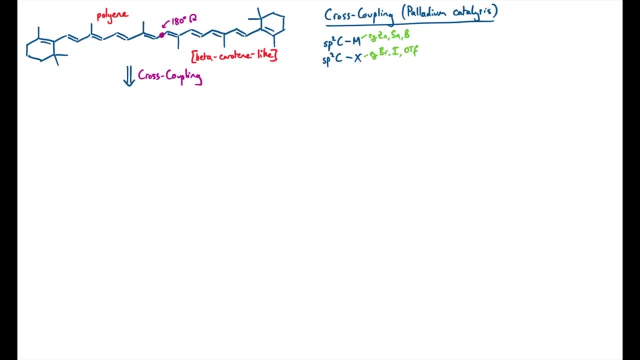 these are probably the most common, reliable ones. So the mechanism for these reactions: we'll start with a species like this that has a leaving group X and that interacts with a palladium zero source, which I'm going to represent like this. it'll always have some ligands of some number. so, just for formality, I'm just going to call that Ln. 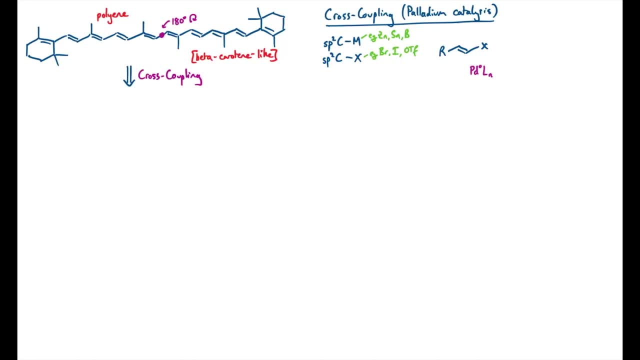 Those ligands can be changed and optimised, but they are actually quite important for stabilising the transition metal complexes and the organometallic intermediates that we're going to draw Now. an inorganic chemist will probably kill me for doing this, but I'm just going to use some. 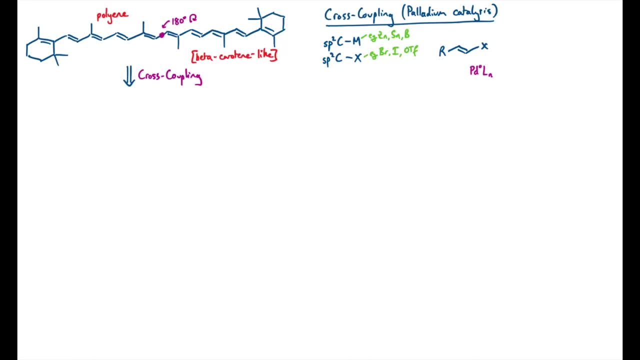 curly arrows to help represent the first step. I'm playing a bit fast and loose with the definition of curly arrows here, but I'm going to use two electrons from the palladium to insert into the sp2 carbon leaving group bond and attach the leaving group to the palladium zero. 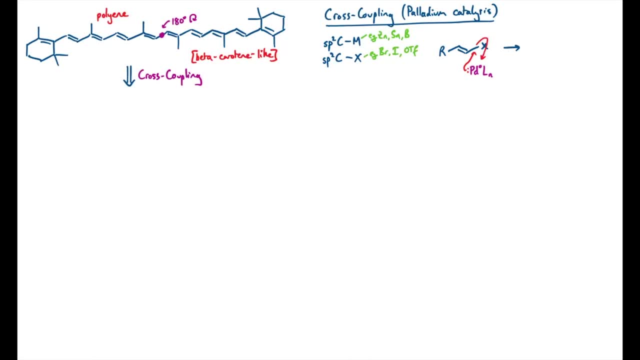 These arrows are just more of a guide for the eye, which is perhaps a helpful extension of the model we're using, As we've lost two electrons from the palladium. the palladium is now in the plus two oxidation state, still got the ligands on it and the leaving group now becomes a ligand. 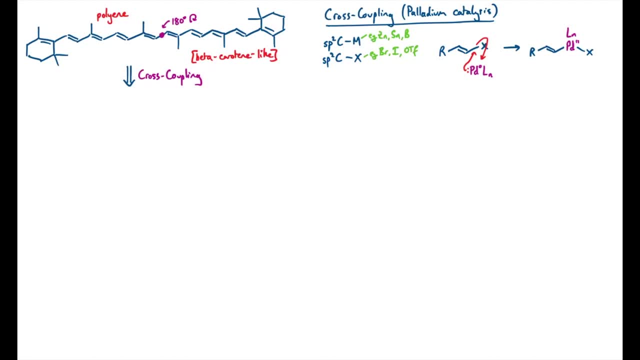 on the palladium itself. so that will give us an intermediate like this. This first step is called an oxidative addition. it's quite a common way of forming an organometallic such as this first intermediate. Now, if this final palladium species comes across, our other coupling partner, 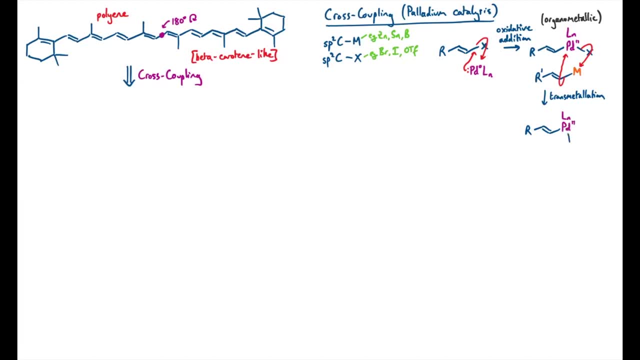 so that's the vinyl metal species. we can do a transmetallation reaction where essentially we're doing a ligand swap, So the carbon originally bonded to the metal will join to the palladium and the palladium will lose its x ligand which can form a bond to the metal. 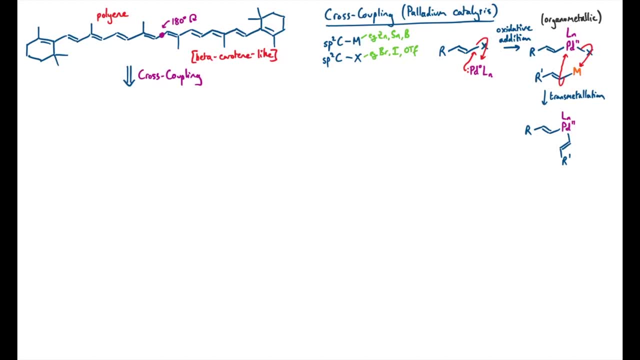 and that explains why we picked some of the things for m and x that we do: because in this transmetallation step we spit out mx and because that's often a salt that can add a huge driving force, enthalpy wise, to this reaction sequence. The final step in the cross coupling: 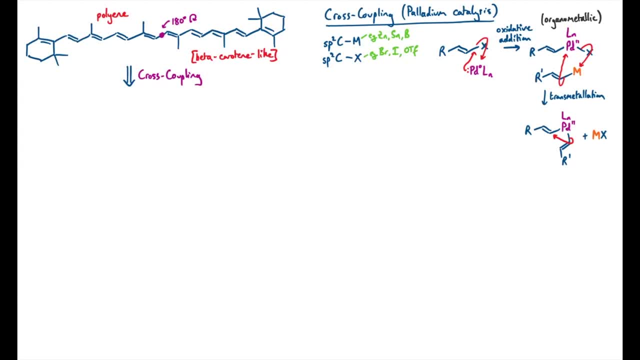 mechanism where the two ligands can combine together, spit out the palladium species, which would dump two electrons back on the palladium and reduce it back to palladium zero. So this is called a reductive elimination and gives us a useful organic product. We now have a new carbon. 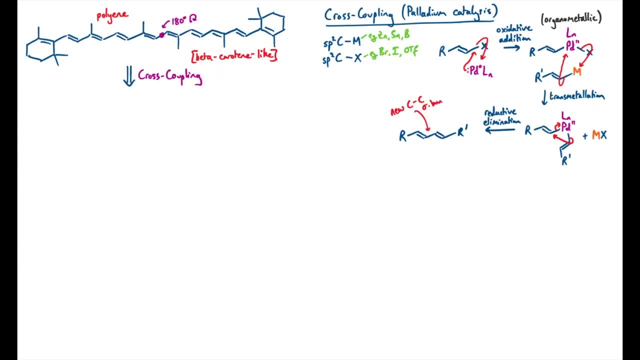 carbon sigma bond. as a result of this process, and importantly, the palladium zero is regenerated and it can go back around this cycle and interact with another molecule of the starting material. So we only need a catalytic amount of our expensive palladium species to get this. 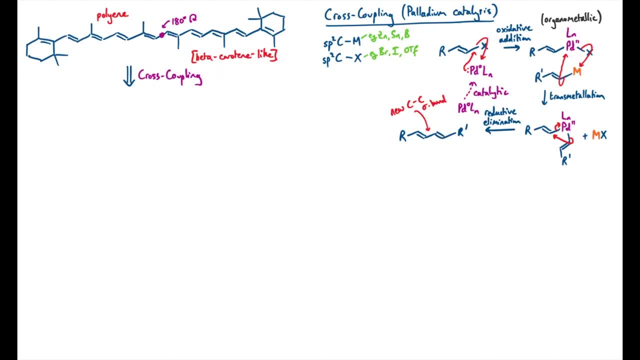 reaction going. in fact, you can get away with quite low loadings if you optimise these reactions. These types of reactions are complete game changers in organic chemistry and revolutionised the pharmaceutical industry. These reactions work really well when you have sp2 carbons involved. 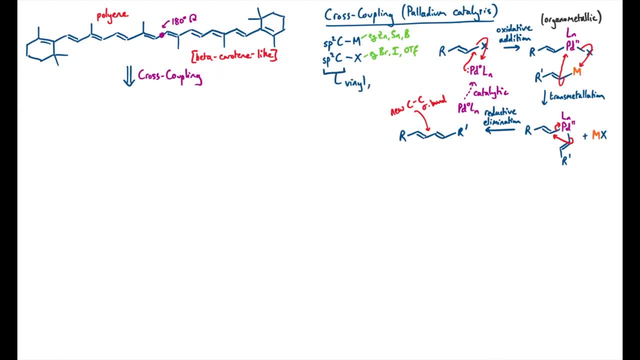 so, for example, I've drawn here vinyl systems, but you could also have aryl systems and others, and there's been lots of research over the last few decades about expanding the reactant scope of this reaction, which has been pretty successful, but that would be a discussion for another time. I 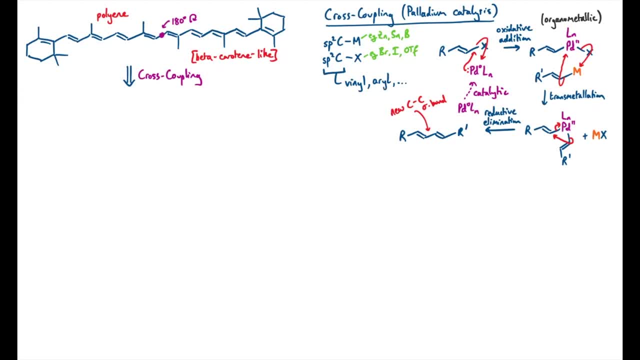 think: Okay then. so back to our analysis. So we've got a couple of different types of molecules here, one of which is called alkyne, and that tells us exactly what components we need. We need to make sure that one side has. 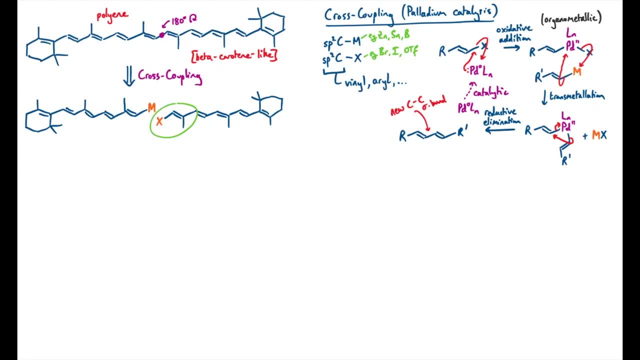 a metal attached to it and the other side has, say, a halide attached to it, but otherwise the structure of those molecules is pretty much the same. All we've done is tweak these end bits, and that allows us to make a major shortcut in our retrosynthesis: We can disconnect both of these. 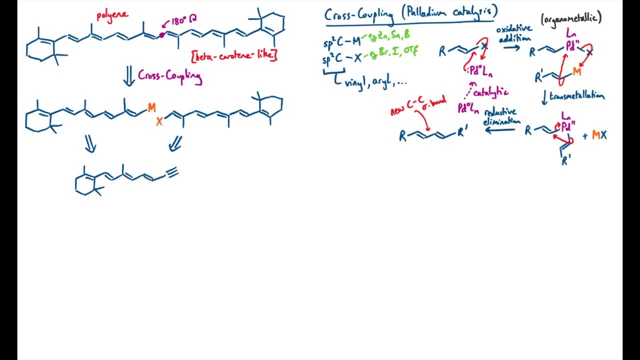 species back to a common precursor which looks like this, with an alkyne at the end, and that's because both of the motifs we require can be made by a carbo-illumination reaction. Now, as this might be a less familiar disconnection, I'll just highlight what the mechanism is thought. 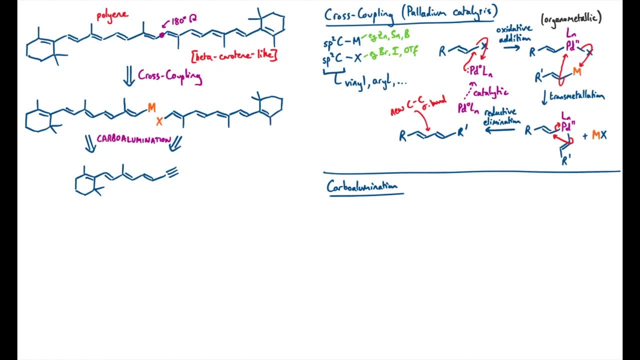 to be here. We're now in the territory where it's pretty tricky to draw curly arrows, as we've got a lot of metals involved here. but this reaction can be very useful, and what we do here is we react an alkyne with trimethyl aluminium and we use another metal. 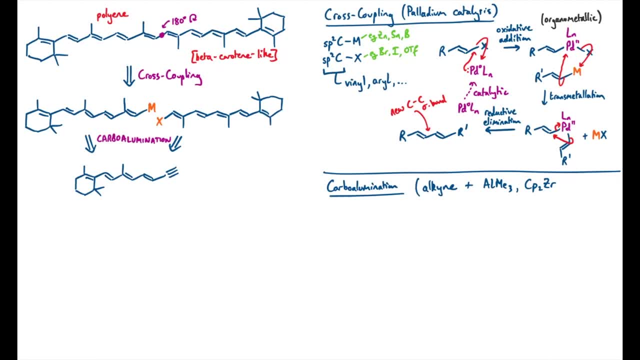 to help catalyse this. We use this dicyclopentadienyl zirconosine type species. in fact, we use the dichloride as a catalyst, So this is like a transition metal sandwich complex, the CP here. 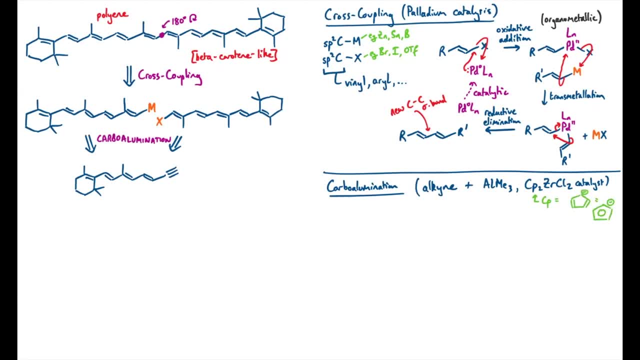 It's just representing the cyclopentadienyl ligand, which usually coordinates via its pi system as one big six pi electron donor. We could represent it as either of these structures, but normally we draw the circle for me, if we're going to draw this out, 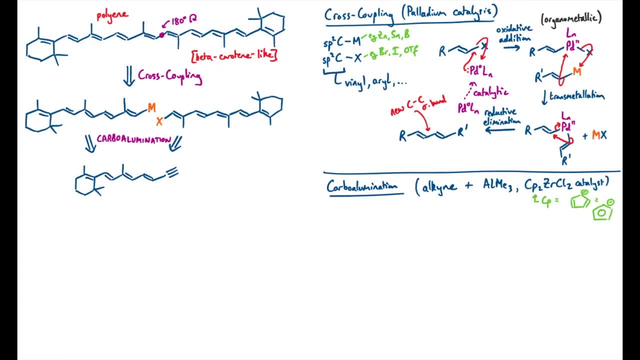 So just to sketch out the intermediates here, so that we can see how this reaction works: the trimethyl aluminium on its own cannot react with the alkyne, so what we do is we activate it by complexation with the zirconium catalyst. 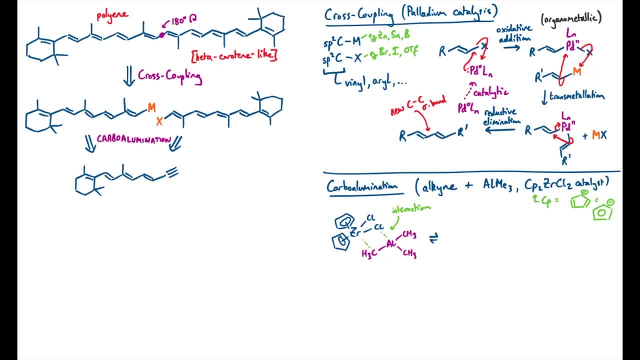 When these two species get together we form some interaction between the carbons and the chlorines with the opposite metal centers, which both have a bit of empty space in their coordination sphere. Now the bonding here can't really be represented by traditional two-center, two-electron bonds. 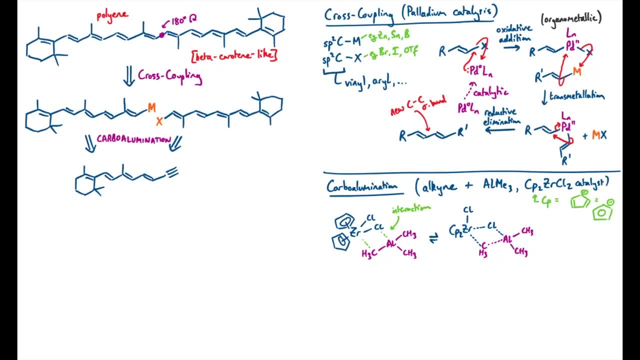 I'm just going to use some dotted lines for now to represent the fact that this bonding is slightly more fiddly, but it's known that this intermediate exists. This complex is fluxional and can rearrange. to use just the chlorines to bridge between the two metal centers and, formally, 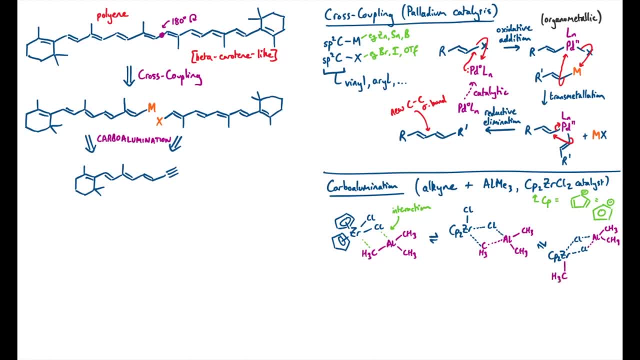 transfer one of the methyl groups onto the zirconium center directly. This is thought to be the key reactive intermediate that we will be using for the two-center. two-electron bonds reacts with the alkyne and we can do a carbo zirconation reaction. that's adding that carbon. 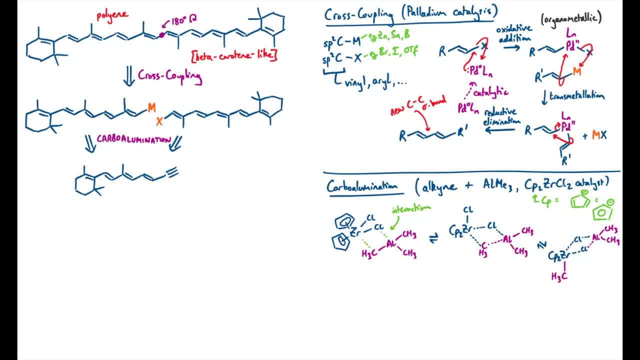 zirconium bond directly across an alkyne, but we might be able to do that in two different ways, so I'm just going to use the example I need in my retrosynthesis. all of this extra ligand stuff up here is very bulky, so the best way for an alkyne to interact with this would be to put its sterically. 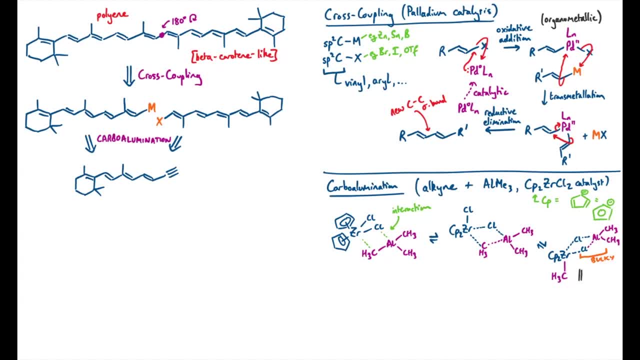 smaller end in towards the zirconium. so I'm just going to use a terminal alkyne here. so this is just arranging on sterics and I could draw some arrows to guide the eye here. the terminal position with the bulky zirconium center will add to the end of the alkyne and at the same time the 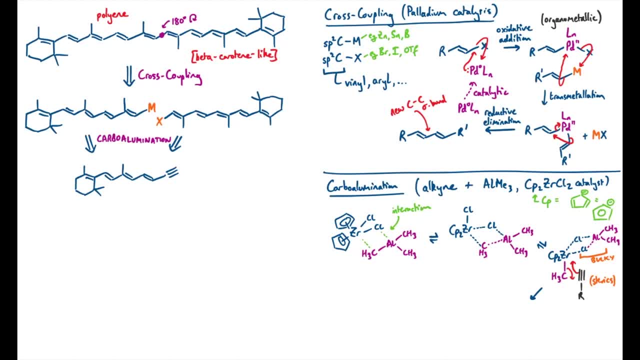 methyl group will transfer to the internal position. this type of process is known as a migratory insertion. so our next intermediate has a methyl group installed on the internal position and the zirconium is just added to the end of the alkyne. now it's known that these ligands can dance around. 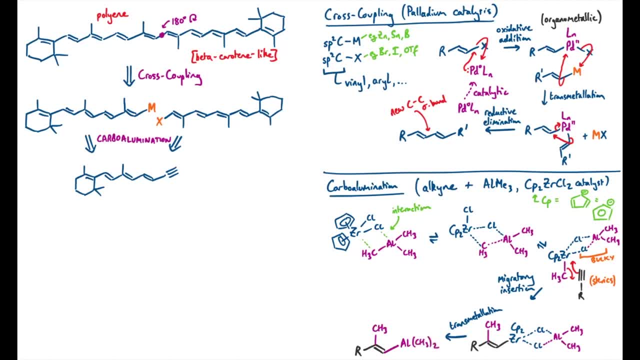 a little bit. in fact, they can do another transmetallation to give us this organometallic, which is known as an allane, because it's an organometallic of aluminium, but in doing so we also release a zirconium catalyst which can then go back. 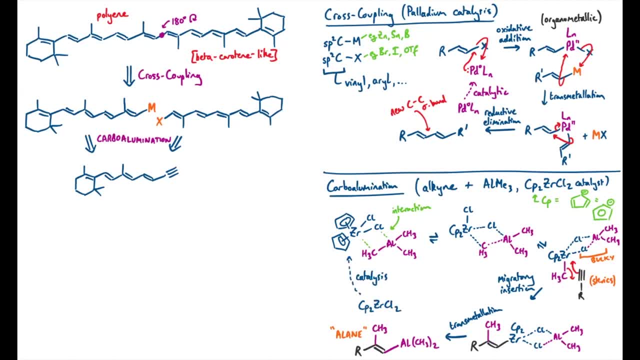 around to the start of this sequence and help out another trimethyl aluminium to add across another alkyne molecule. now this allane is getting quite close to being a bit like a grignard and it can react as a nucleophile with strong electrophiles to form all sorts of species and 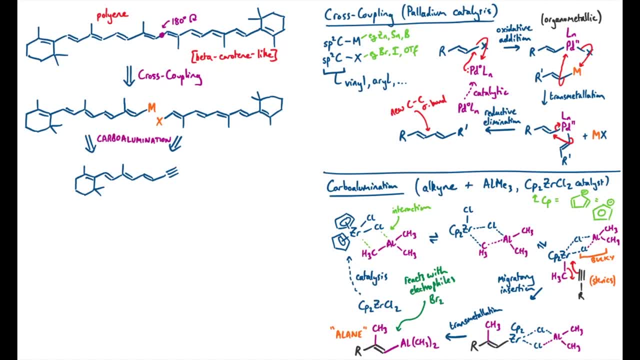 importantly for us. some of the things that this can react with is to directly attack something like bromine or iodine and that will form new carbon halide bonds. or we can react with metal centers, say as part of a chloride salt, to form a different organometallic of our choice. 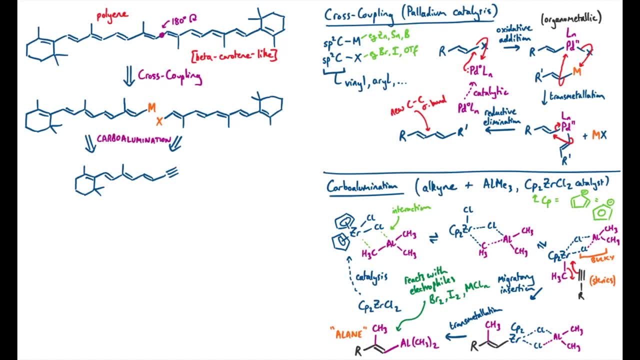 so what we're going to do in our retrosynthesis is to split our starting material, alkyne, into two, make the allane and trap it out with a different thing. fifty percent of it can get a halogen and fifty percent of it can get a metal. we could use something like zinc chloride in this case. 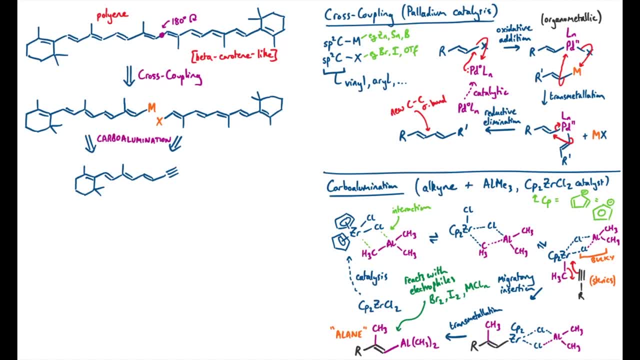 okay then that's enough of a detour, let's go back to our retrosynthesis. well, we need to find another disconnection point. there's still loads of sp2 to sp2 carbon bonds here. i'm just going to do another cross coupling across here to sort of roughly go in the middle. 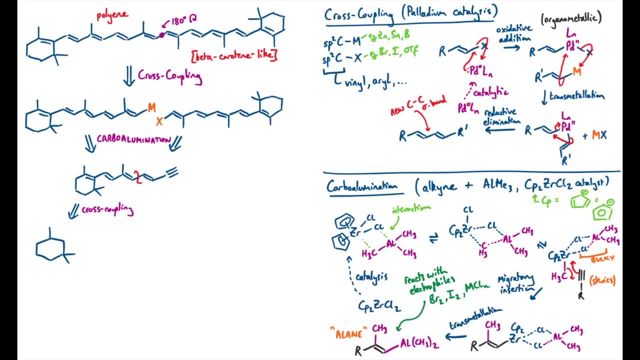 so doing, another cross coupling reaction would take me back to a species like this. so i'm just going to pick this side as the one with my metal and i'm going to need another component with a halide, perhaps something that looks a bit like this: the alkyne fragment, actually. 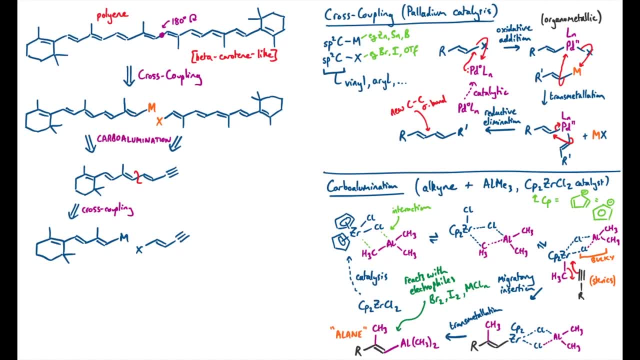 has a pattern that lends itself to another cross coupling type reaction if i disconnect across the middle. this is an sp2 carbon bonded to an sp carbon. this can be disconnected using a sonic coupling. this is very similar to the other cross couplings, although we form the organometallic. 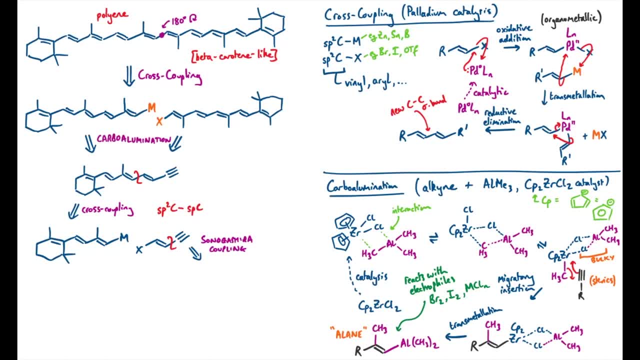 species in situ, largely because an alkyne has an acidic proton on it which the sp2 carbon species didn't have. this will take me back to a fragment that looks a bit like this, perhaps with two different halides on there. there is a reactivity window between bromides and iodides that we can 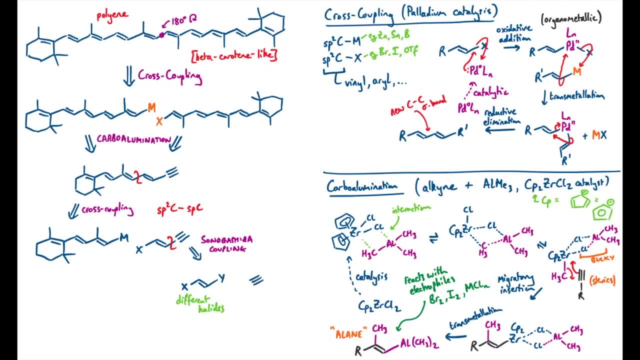 exploit here and we're also going to need acetylene. now there's a bit of a problem here. firstly, acetylene is horrible to work with. probably want to totally avoid that. but also if we end up with dihydroxyate hierodyl, we're not careful. the acetylene is symmetric and has acidic protons on either side, So if we're not, 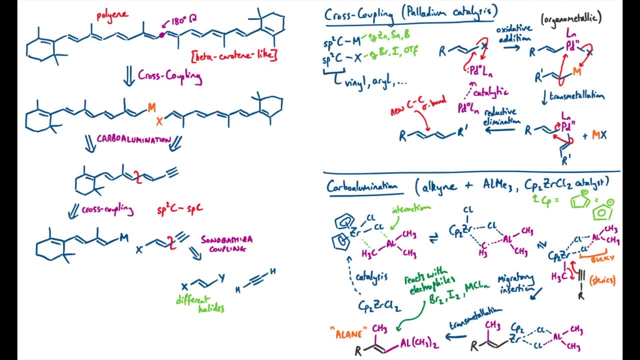 careful. we'll do a sonogashira coupling on both ends of that alkyne and make a product that we don't want. So we're going to need to block one end of it with a protecting group and a very sensible one to use just a trimethyl silo group and we can just use this TMS acetylene. This is a 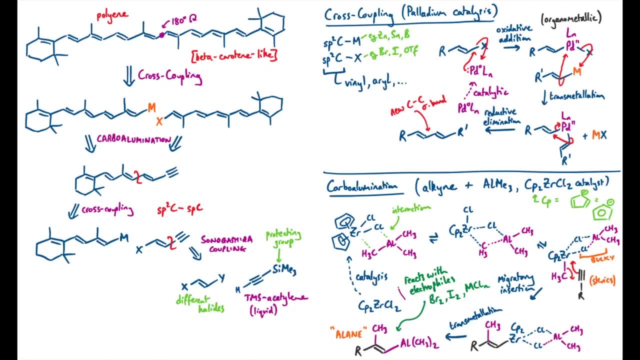 much friendlier reagent to use in the lab. In fact, it's quite a stable liquid that you can just store in your fridge, Much easier to deal with than an explosive gas. Even if you have bare acetylene in solution it's a safety nightmare. Strong recommend to avoid it if you possibly can. Okay, and to finish, 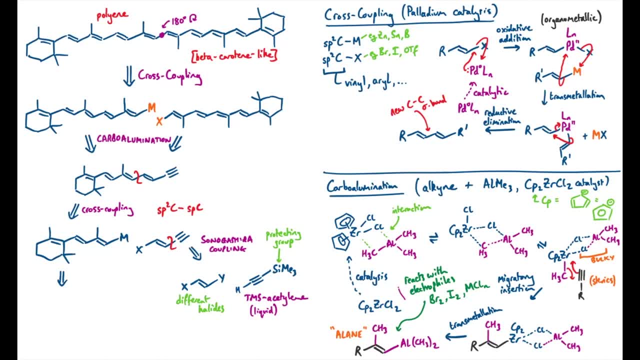 off my retrosynthesis, I identify that I have the same pattern that I had before, so I can do another carboillumination. to take me back to an alkyne. We could play the same game as before with the cross couplings, but actually I think it might be a good idea to make this alkyne in a slightly 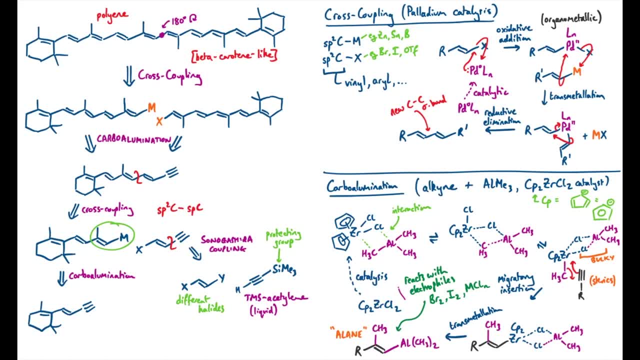 different way, because I happen to know some cheap and readily available starting materials that are very close to the alkyne. So I'm going to use this alkyne to make this alkyne, This molecule that I've drawn specifically this ketone. this is an incredibly cheap starting. 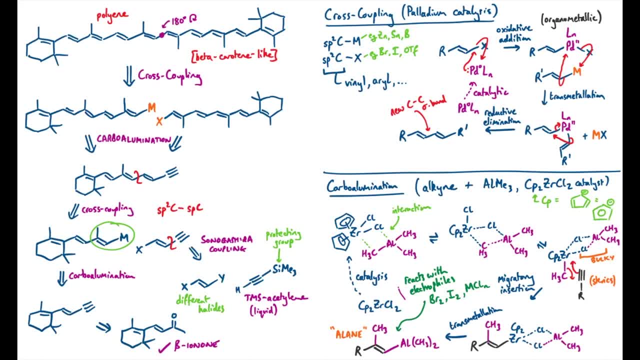 material that comes out of terpene biosynthesis, and in fact, it's one of the main reasons why roses smell like they do, So this is a scent molecule. Being aware of things like this can really help push your direction in syntheses, and I'm just going to go on to the next slide to really 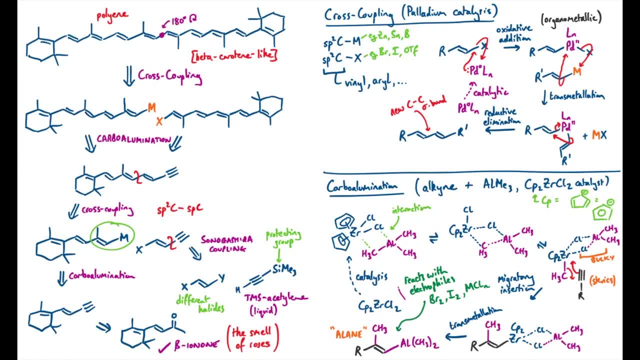 emphasize why it's a sensible idea, as a chemist, to have an awareness of common molecules in nature, because it can make your syntheses way easier and much less time consuming. I'll also show you what reagents we need to convert that methyl ketone to the alkyne. but you might be able to see that all. 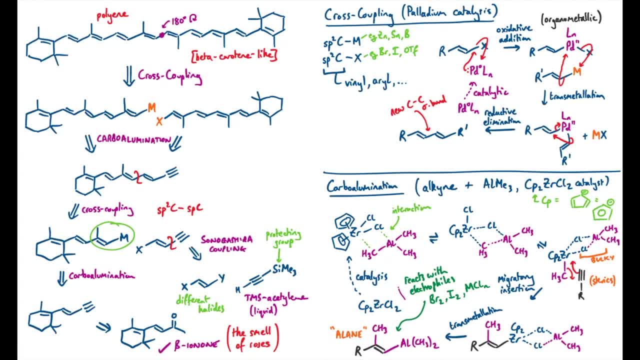 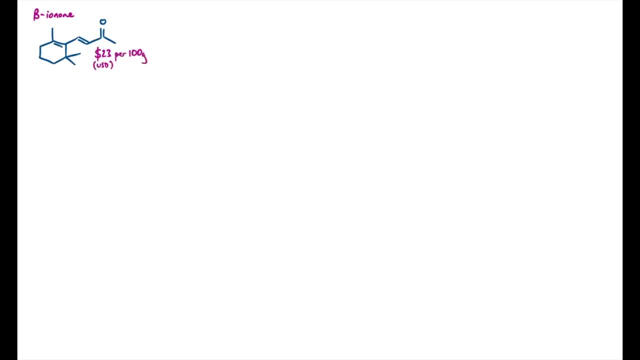 we need to do is lose water from that molecule, so we just need to engineer a dehydration reaction. Okay then, so this is my beta-ionone As I'm recording this video. this is currently available from chemical suppliers at 23 US dollars per 100 grams. Now, 100 grams of this molecule is about 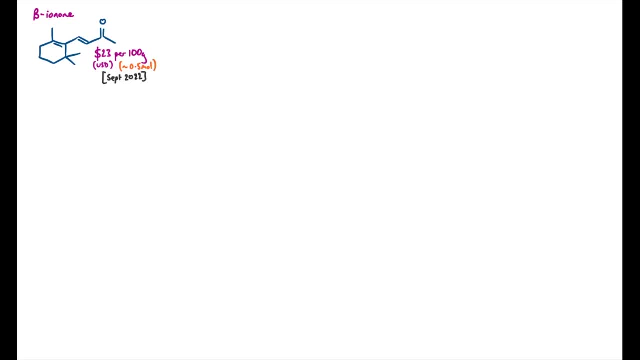 half a mole, so you're getting quite a lot for your money there. Just as a fourth exercise, I thought we could just have a look at the retrosynthesis of the beta-ionone To show that actually it would be quite a lot of effort to try and make this from smaller molecules. 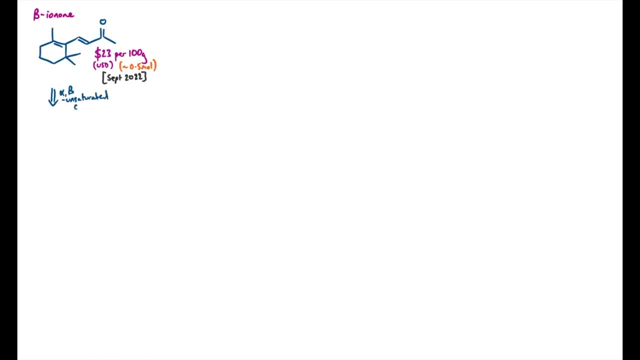 First thing I would do is disconnect across the alpha-b2 unsaturated carbonyl like this. Now, those reactions are easily done by aldol condensation or Wittig reaction. So in this case a Wittig reaction will probably be quite easy, because this phosphorine is cheap. 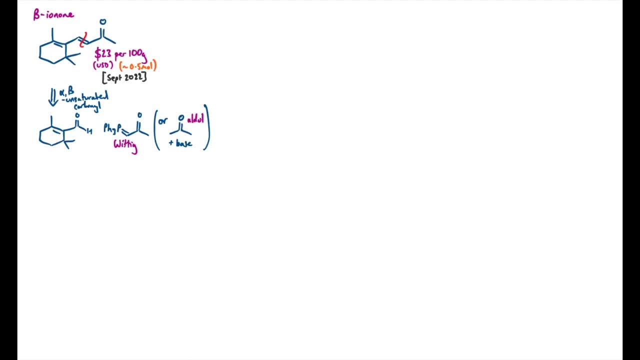 and readily available. but I think we could probably get away with the aldol as well. We just might get a few more side reactions, but there's no denying that would be a cheaper route. One thing we might notice is that there's a cyclohexene. That's a bit of a trigger for doing. 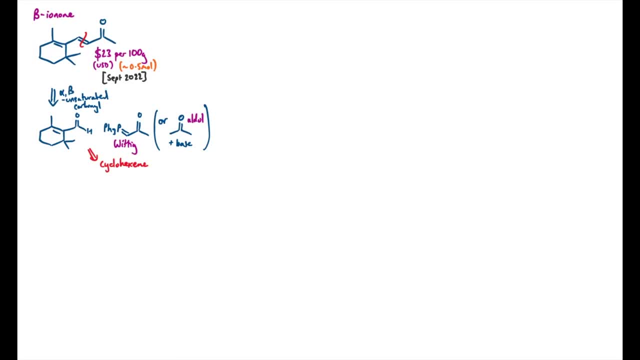 a Diels-Alder reaction. but actually, if we look at what the intermediates we'd need, well, it's not going to work. We'll have an electron deficient diene and using ethylene as a gas there it's not particularly operationally easy. So I'm going to discount this route. That Diels-Alder reaction is. 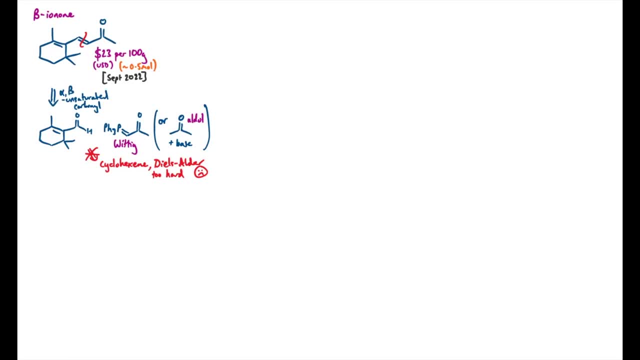 too hard. So the alternative disconnection would just be to cut across here and notice that it's an alpha-b2 unsaturated carbonyl again. So therefore I could do aldol or Wittig. The Wittig reaction will be quite tricky to do here because it's intramolecular, so you need to make the illid. 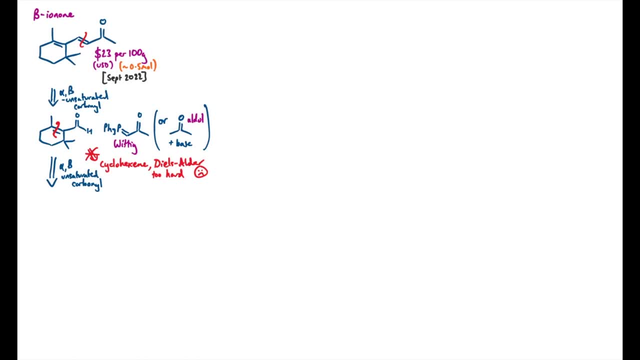 on one side of the molecule and have your electrified reaction. So I'm going to do a Wittig reaction here because it's intramolecular. so you need to make the illid on one side of the molecule and have your electrophile on the other, Or it would just be much easier to here to do an. 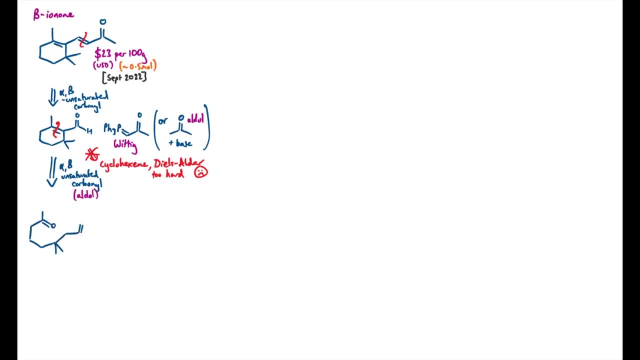 intramolecular aldol reaction, and that will take us back to something like this, which looks simple enough: We've got the functional groups in the 1, 2, 3,, 4,, 5, 6, 7 relationship and they're just. 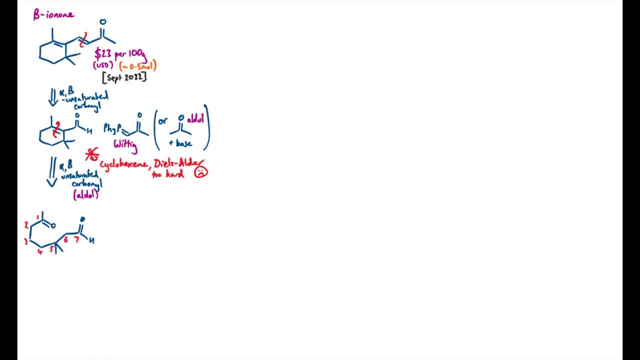 carbonyls. so perhaps we can use some standard chemistry to make this linear precursor. but we do actually have a major problem here. We've got some major control issues. To do the aldol that we want, we must enolise at carbon 6, but unfortunately there are other enolised. 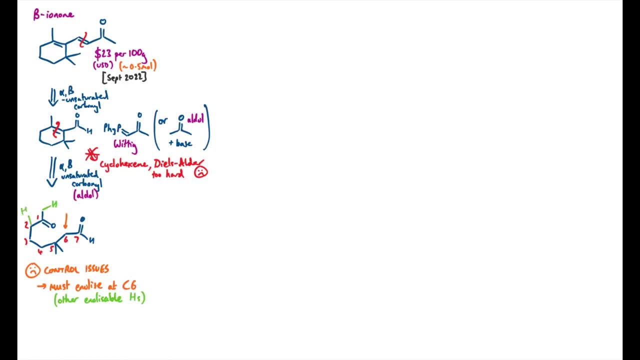 hydrogens, In particular these ones I'm just highlighting in green, and so we'd have to be very careful. we got the one we wanted. The one at the end here on the other side of the methyl ketone is the most sterically accessible one and also, if we happen to form the enolate at position. 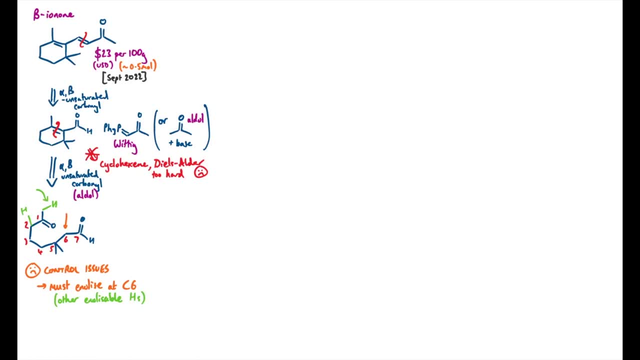 6, it's perhaps a less reactive enolate because it's right next to these methyl groups which would add some steric bulk near the nucleophilic centre. Now I think we're okay to discount the reaction between these two centres in purple, between an enolate of that methyl ketone, because 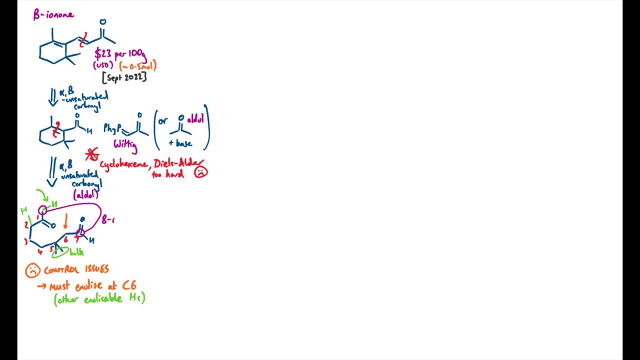 this would be forming an eight-membered ring, and the eight-membered ring will be much less favourable as a cyclisation than any possible six-membered rings. but the one thing we really can't discount is the reaction between centre 2 and centre 7 like this: This reaction will go on. 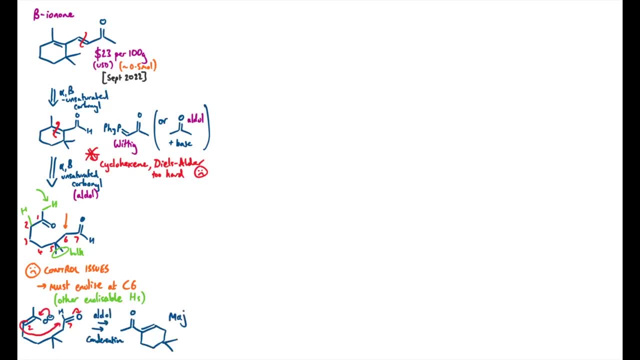 to form this aldol condensation product, which is probably the major product. That's because it's got the better nucleophile, the sterically less hindered enolate reacting with the more electrophilic carbonyl in the aldehyde, again for steric reasons. So we're not going to get what we. 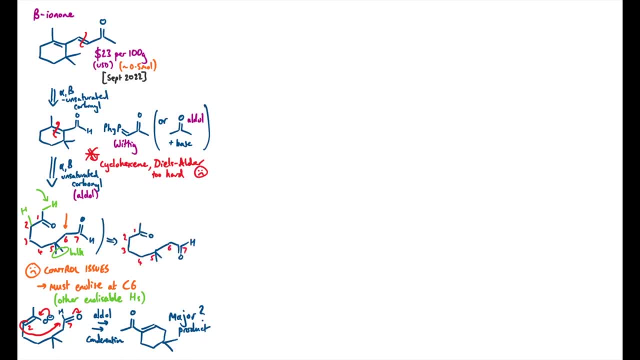 want if we try to do this. Perhaps one way to do this would be to edit the starting material so that we definitely get enolisation at position 6.. I mean, common ways of doing this would be to add a beta ester and then later decarboxylation. but already we're making our lives way more complicated. 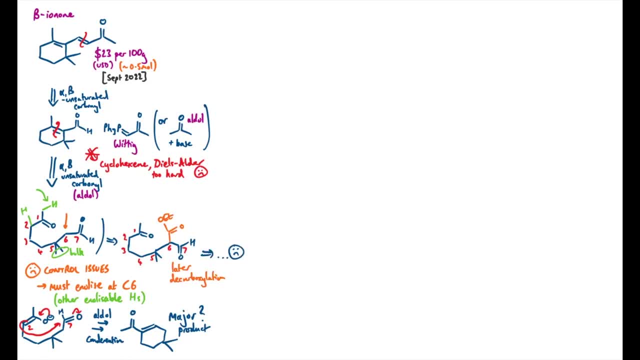 than necessary, and I think we should abandon this route Now. it's not that we can't make this molecule, but our target ionone is available for very cheap, whereas our time is probably more valuable, and we're already making a multi-step synthesis here, which will take a while. There is. 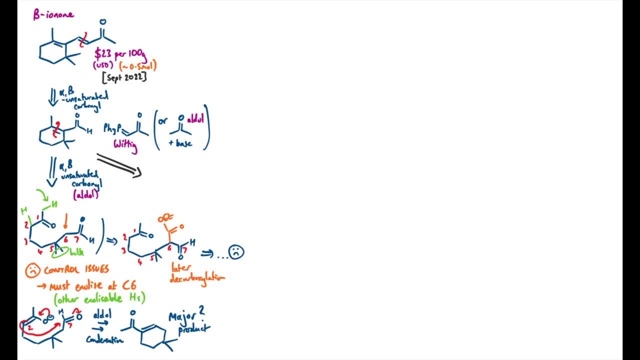 a classical disconnection here, which is that rather than using an aldol reaction, I'm just going to intercept the alpha beta unsaturated intermediate here with a star and just make that C-C double bond by a different type of elimination reaction. We don't have to use an aldol condensation In. 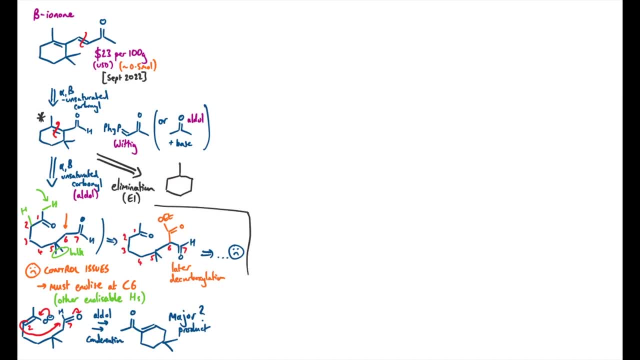 fact I'm going to give E1 a go. If I disconnect back to this carbocation, it would be possible for me to use carbocation chemistry to make this molecule. For example, I could do a disconnection that looks like this and move my tertiary carbocation to the other part of the molecule. I 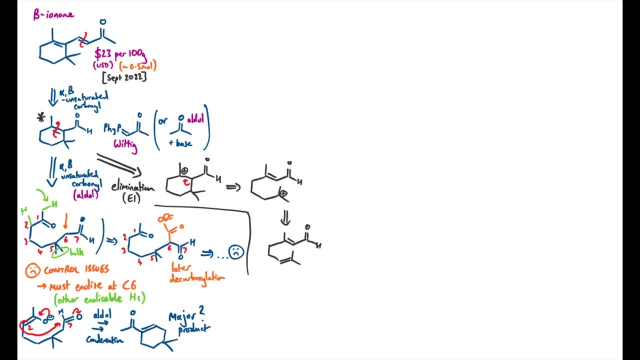 would use that carbocation by protonation of that alkene and then we're sort of done Just going backwards. that would be, for example, using something like HBr as a strong acid. We would react with the most electron-rich alkene, the better nucleophile It'll attack. the H plus this. 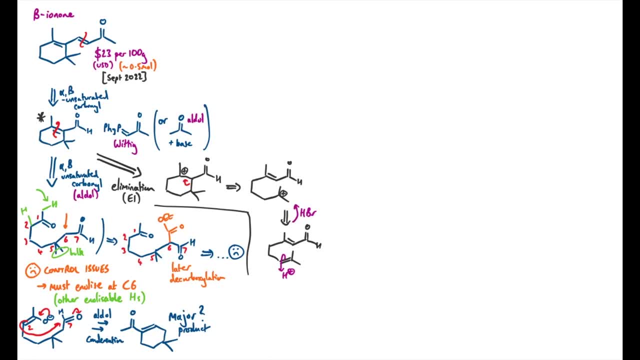 way, just obeying the Markovnikov rule, to give me a carbocation which then could do an intramolecular cyclization, Then finally have that proton picked off by an external molecule to leave me with the best possible C-C double bond. That would be the one that's conjugated with the carbonyl and I. 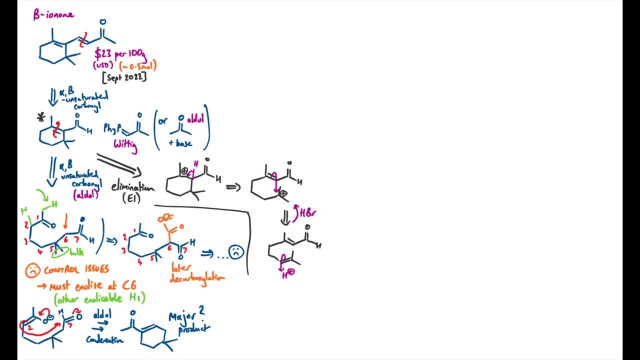 think that's a decent level of control, But again we're going around the houses here. This is a bit of a waste of our lab time. If I wanted to disconnect this, well, I could do an aldol condensation on that. alpha beta unsaturated. 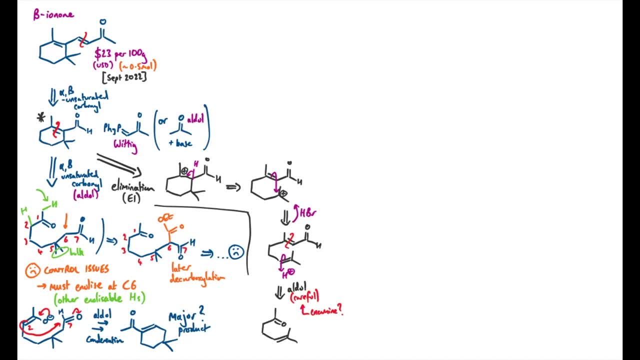 carbonyl. We'd have to be careful of that aldol because we'd be proposing using the enolate of an aldehyde. So maybe we could use an enamine or something there, Although it'd be pretty easy just to use a vitic reaction instead. Then this final species should be fine. We can just use some. 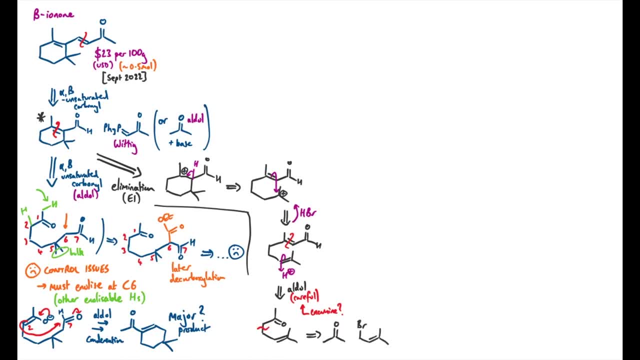 enolate alkylation chemistry here to do SN2 on this pre-null bromide which is cheap and readily available. Right, so that was really quite a big detour to try and make my point, but I hope it was helpful to think about things like this In my synthesis of my original polyene for this video I'm going to. 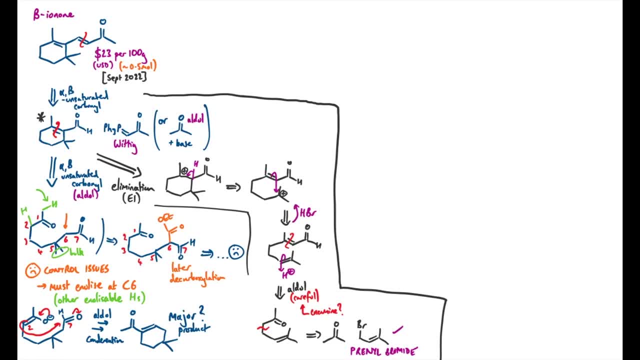 buy in the beta-ionone and just be done with it. I need to do a dehydration reaction. Well, it's going to be a bit cheeky. I'm going to use the enolate and dehydrate that. So I'm going to use LD8 at 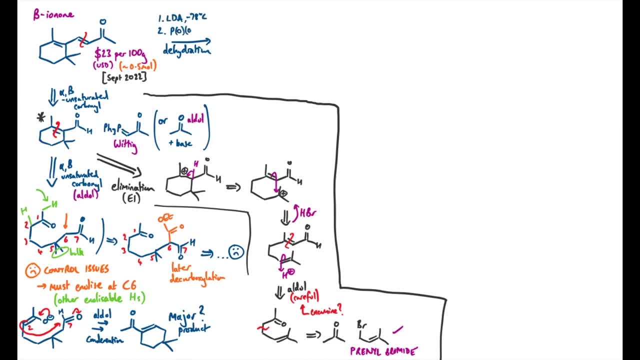 minus 78 degrees to form the lithium enolate and then react it with this phosphoryl chloride. I'll just draw the mechanism in a second. That species will react preferentially with the oxygen end of the enolate because the phosphorus-oxygen bond is so strong compared to a phosphorus chloride bond. 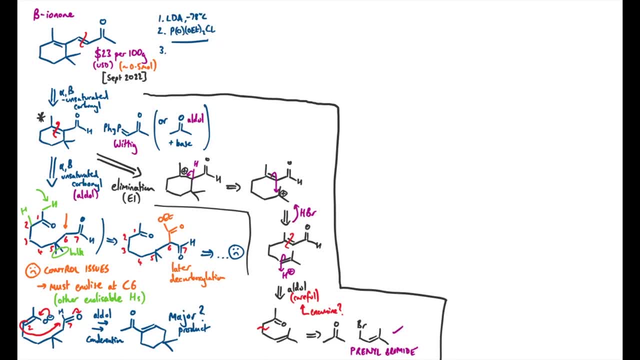 And then finally, if I use a little bit more base, just using LDA again, I'll be able to eliminate off a leaving group. So just sketching out the mechanism there: Started off with the methyl ketone. I'm going to treat it with LDA to form the enolate. The oxygen gets activated as a leaving. 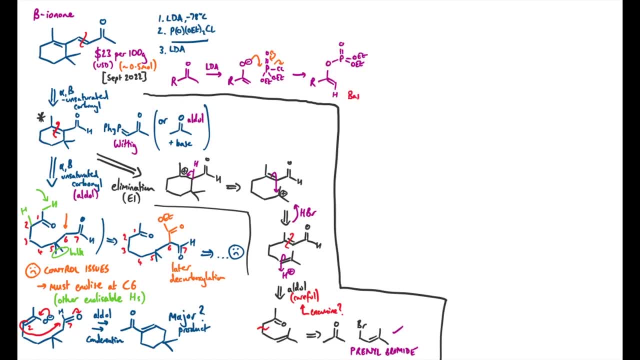 group, and then our second molecule of base can come in and do an E2.. That will form another strong phosphorus-oxygen double bond. This sort of chemistry is quite common in the synthesis of nitriles, but you can also use it to make alkynes as well. 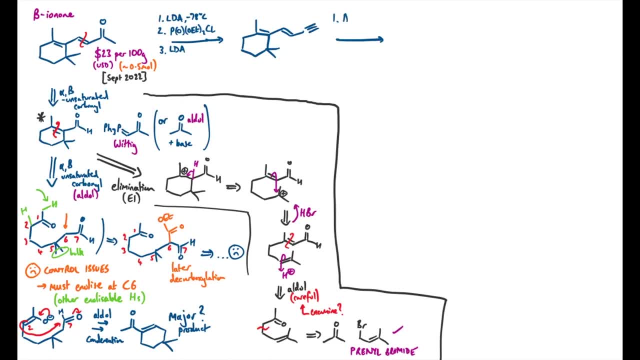 Okay. so next I'll do my carbo-illumination chemistry, So that uses trimethyl aluminium and the zirconium catalyst, And what I'm going to do is I'm going to make the allane and then just trap it with the metal of my choice. I'm just going to use zinc dichloride, because I think that will work. 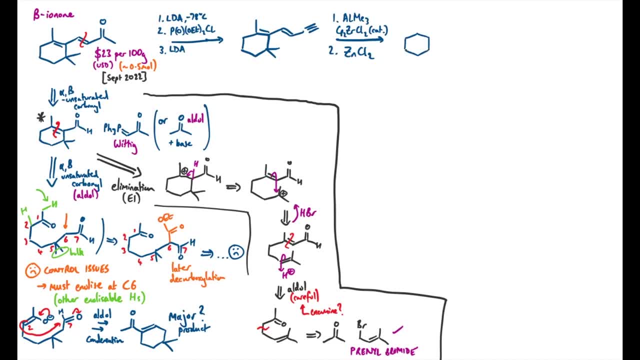 pretty well in the rest of this synthesis, Although there are plenty of alternatives you could use there. That will give me this organozinc species and that's ready for my first cross coupling reaction. We'll just hold that there for a second. The other component I needed was something like this with: 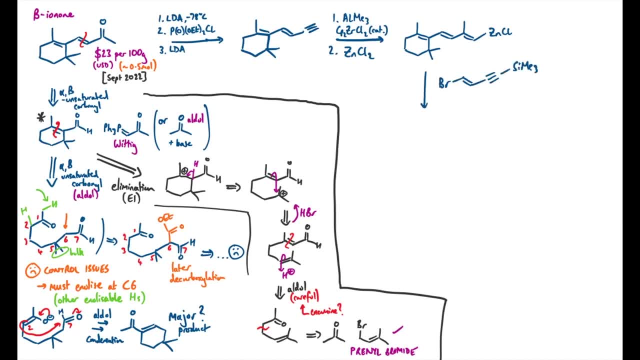 the silicon protecting group. The cross coupling needs a palladium zero source. So quite a common one would be this one: Palladium DBA, And we only need the catalytic amount of that. We need to make sure that palladium center has the correct number of electrons at each of its steps. So in fact we 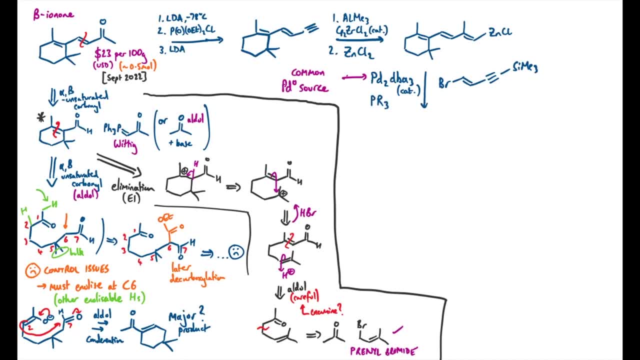 need to make sure that there's a phosphine in there as well. This is all to do with stabilizing that transition metal in all the organometallic reaction steps, And you could optimize this using different R groups on those phosphines. So that's what I'm going to do, And then I'm going to go back to the 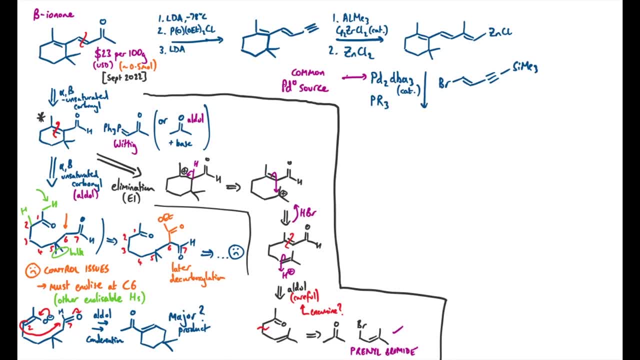 R groups, A common starting place would just be to use triphenylphosphine, So I'll suggest that for now. Okay, what we're proposing to do here is actually called a Noguchi coupling, And that's because we've used an organozinc. Organozincs are really fast at transmetallating, So this reaction. 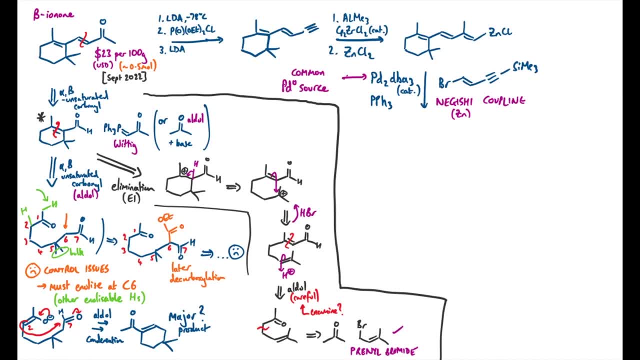 should work pretty well. You might not always be able to use an organozinc, of course, because they can have Grignard-like behavior as well, But luckily in our molecule here we don't have any other functional groups that wouldn't be tolerant to that. We can make our coupling partner from. 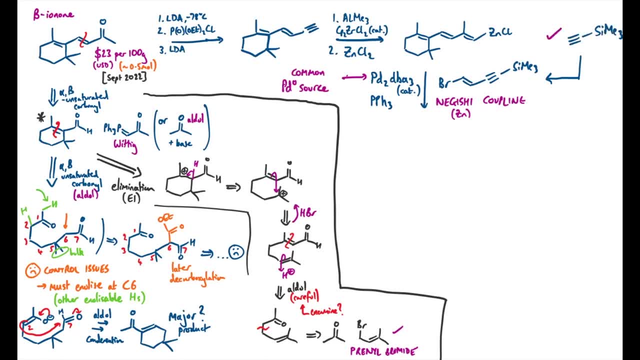 TMS acetylene, which is available, and just react that as a ton of Gashira coupling. This is another type of cross coupling. Essentially we need a palladium zero catalyst, We need some sort of phosphine, We need a copper iodide catalyst, We need a weak. 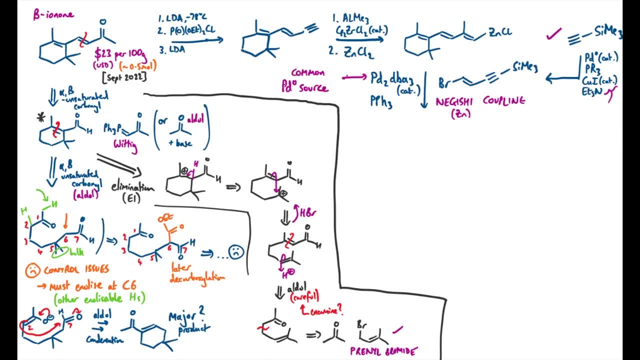 base in triethylamine. These two actually make the coup rate from the alkyne. And then we need a coupling partner. Well, I think we can just use this disubstituted alkene. The carbon iodide bond will react much faster than the carbon bromine bond in these sorts of conditions, So we should 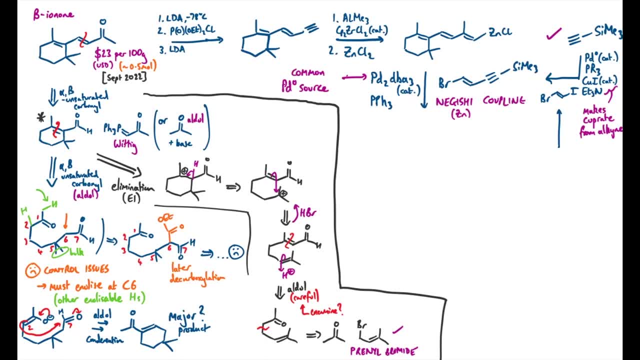 be able to get chemoselectivity there. Now this guy's actually available, But if you're interested, this is actually made from acetylene. Again, not necessarily my favorite with HBR and IBR. This is presumably going via some sort of iodonium species which are getting opened by a. 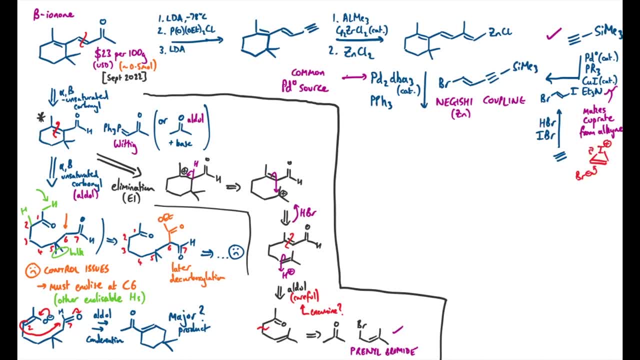 bromide, But with all of those reagents I'm happy to let someone else do that for me and buy it in Pretty much, just from a safety perspective. all of those reagents are horrible. Okay, so after the coupling reaction, I have this intermediate here. We no longer need that. 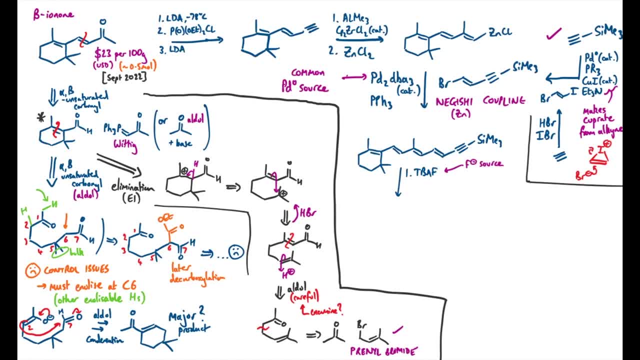 silyl protecting group. so I can just take it off using TBAF. That's an F minus source, Pretty good for forming bonds to silicon and convince it to release our alkyne. And next I need to do the carboillumination reaction again, So that's trimethyl aluminium under zirconium catalysis. 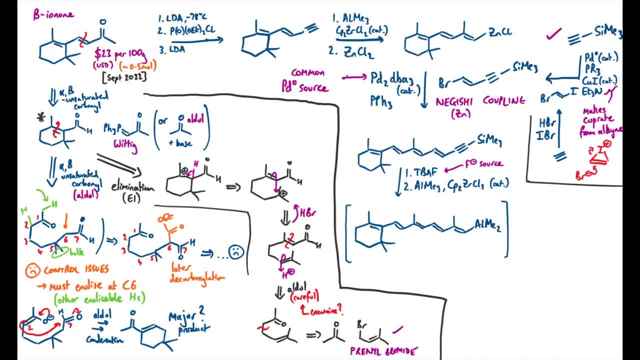 Okay, and that will give us this allane. So what we said we'd do is we've made half of this allane in one flask, which we would then go on to treat with zinc chloride, And that will give us the organozinc compound like this, just abbreviating all of this to R, And we can react the other half. 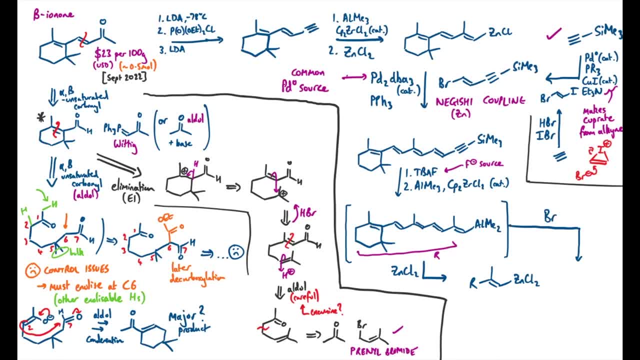 with a halogen, let's just say Br2.. And that will give us the coupling partner that we need, like this. And then, finally, we can do another Nagishi coupling using the palladium source again and the phosphine, And that will get us to our product. 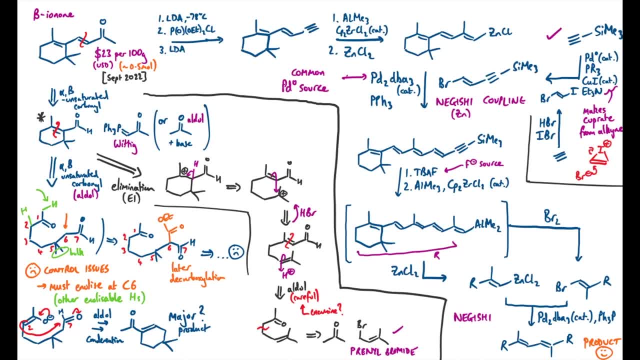 So I made this video using some more modern chemistry than maybe in some of my other retrosynthesis videos. There are certainly lots of other ways of making this molecule like, for example- I could have used lots of Wittig reactions, But this catalytic. 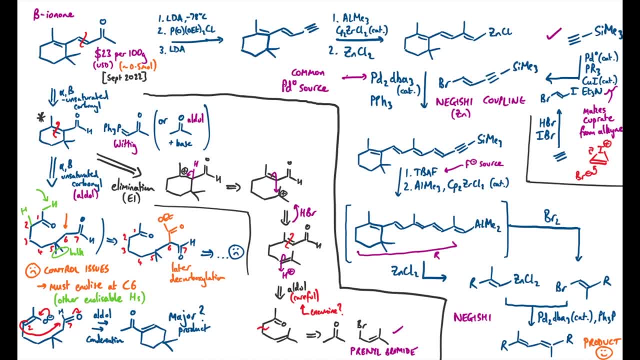 method will generate a lot less waste and should be pretty easy to actually do in the lab. 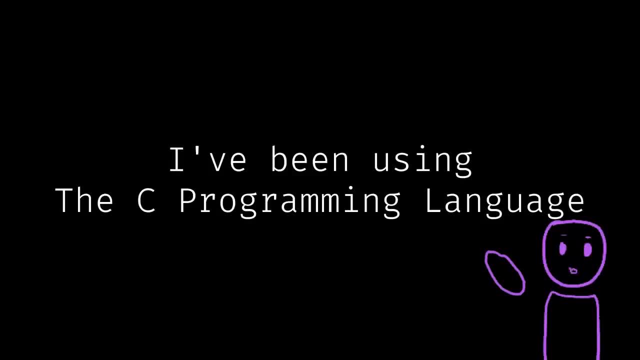 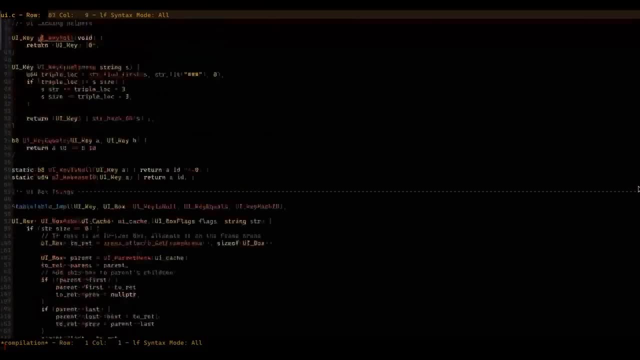 Hey guys, For the past two years I've been using the C programming language for almost all of my projects. This video is about my journey through being completely clueless to relatively okay at the language. It all started when I was looking into how a compiler was made and was recommended. 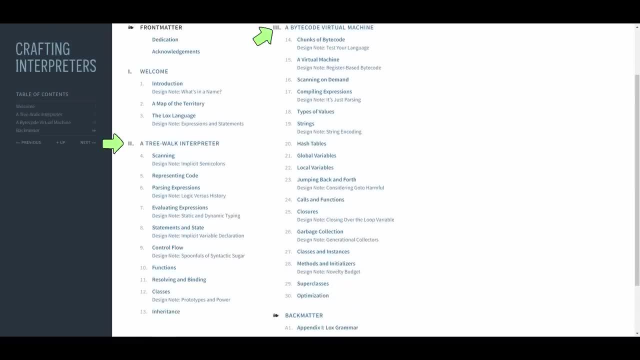 the Crafting Interpreters book. The book is divided into two major sections, both for making an interpreter for the same language, but the first section used Java and the second used C. I was pretty okay at Java at the time, so I followed along and got to the same conclusion.